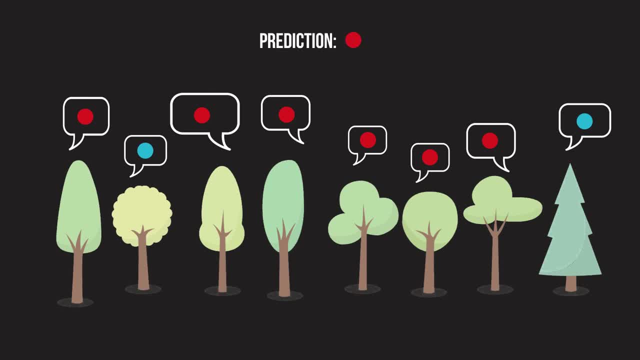 tree spits out a class prediction, and then the class with the most votes becomes the becomes the output of the random forest. In the case of regression, a simple average of each individual tree's prediction becomes the output of the random forest. The key idea behind 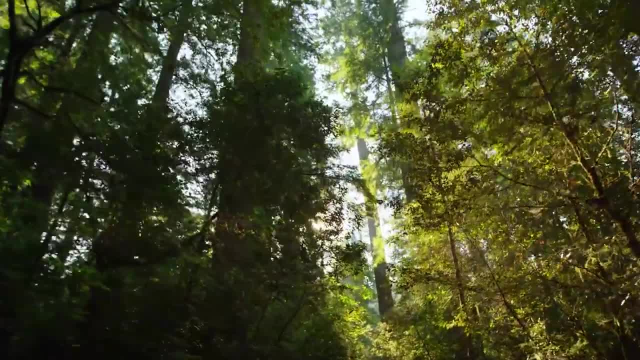 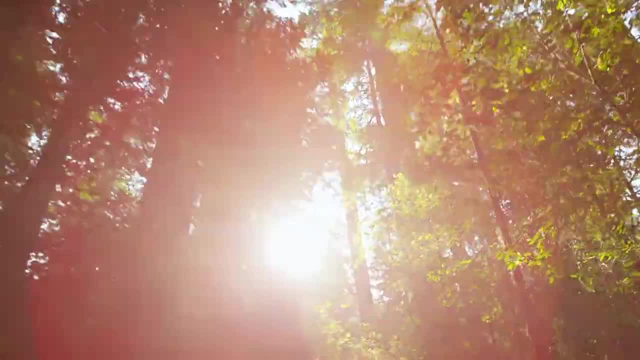 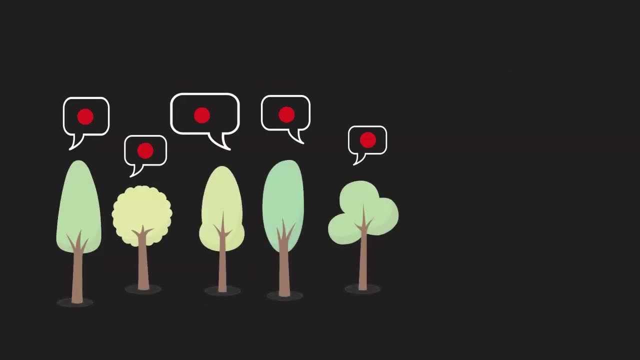 random forests is that there's wisdom in crowds. Insight drawn from a large group of models is likely to be more accurate than the prediction from any one model alone. Sounds simple enough, right, Sure, but why does this even work? What if all of our models learn the exact same thing? 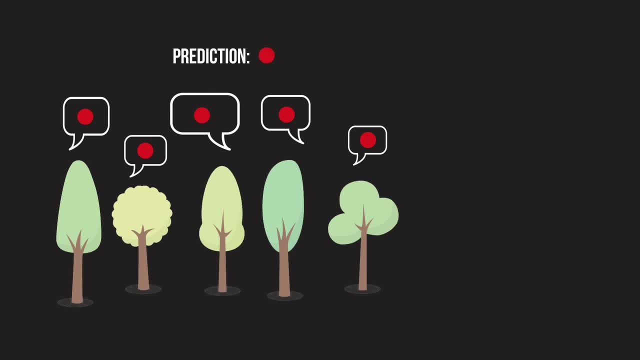 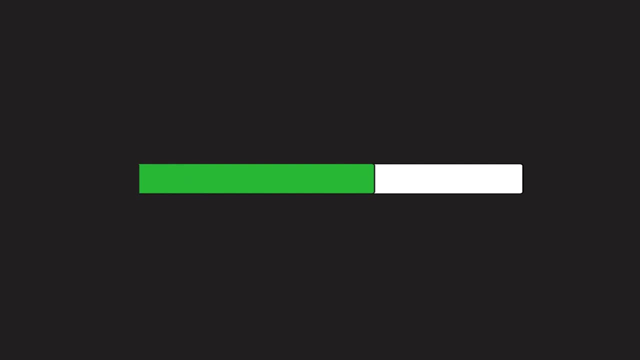 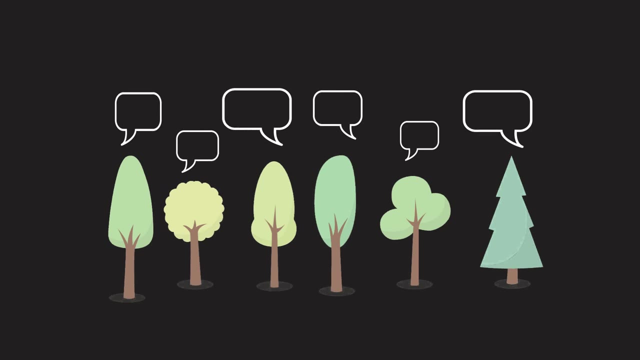 and vote for the same answer. Isn't that equivalent to just having one model make the prediction? Yes, but there's a way to fix that. First, we need to define a word that will help explain Uncorrelatedness. We need our decision trees to be different from each other. We want 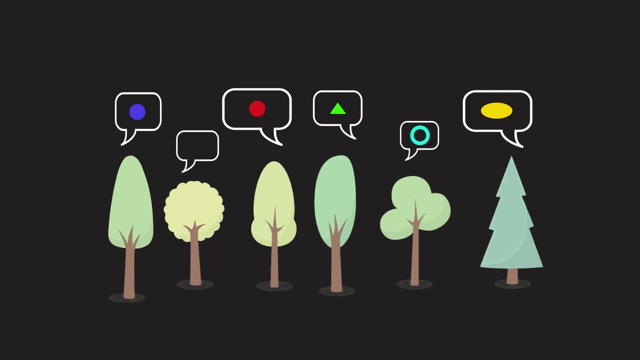 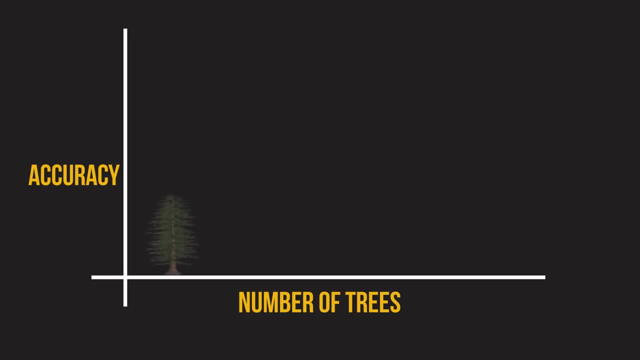 them to disagree on what the splits are and what the predictions are. Uncorrelatedness is important for random forests. A large group of uncorrelated trees working together in an ensemble will outperform any of the constituent trees. In other words, the forest is shielded from. 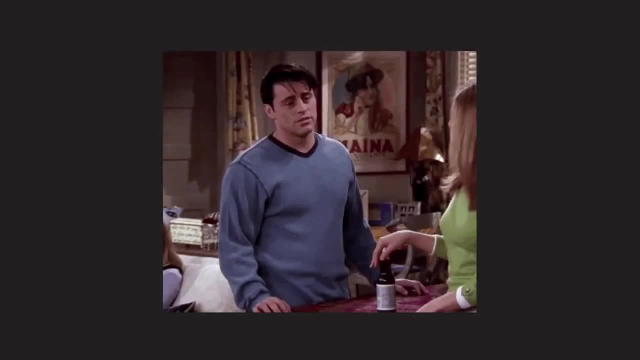 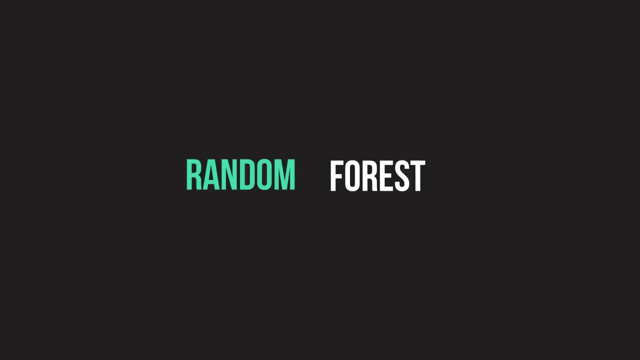 the errors of individual trees. So how do we ensure our trees are uncorrelated? There are a few different methods to do this. As you learn these methods, try and see if you understand what makes a random forest random. The first method to ensure 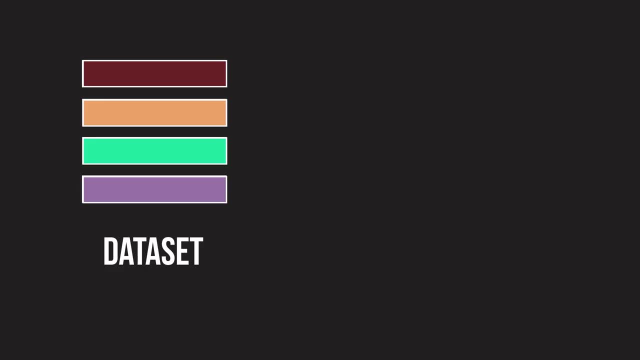 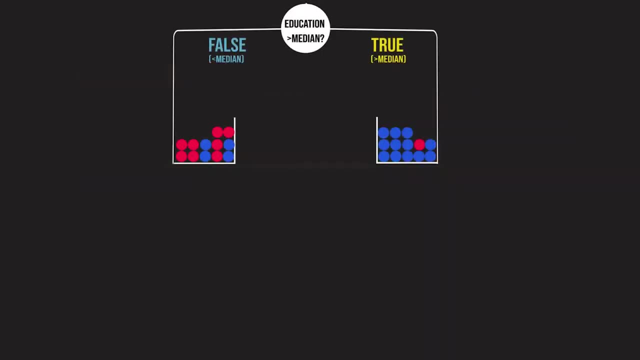 uncorrelatedness is called bootstrapping. Bootstrapping is creating smaller datasets out of the training data set through sampling. Now, with normal decision trees, we feed the entire training dataset to the tree and allow it to generate its prediction. However, with bootstrapping, 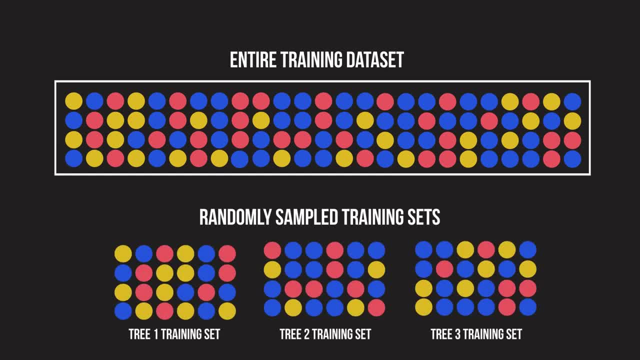 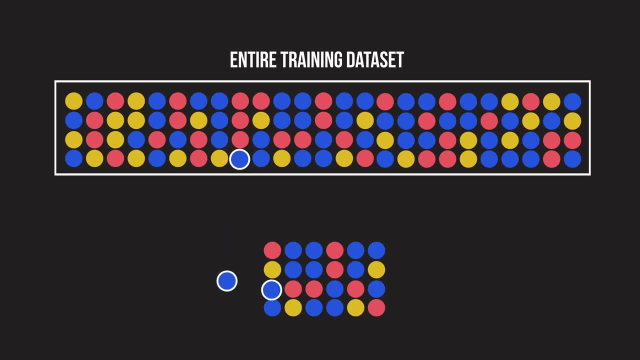 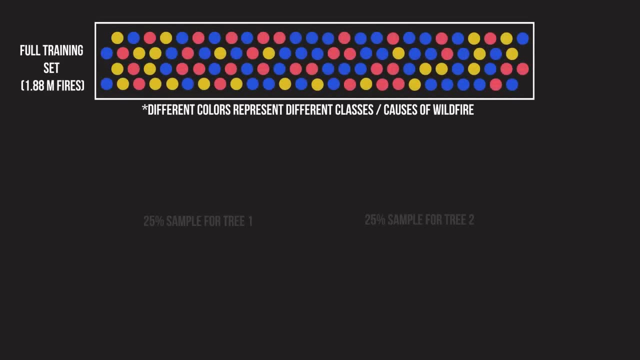 we allow each tree to randomly sample a subset of the training data, with replacement resulting in different trees. When we allow replacement, some observations may be repeated in the sample. In our dataset we have 1.88 million wildfires but we're only going to show, say, a random 25% subset of those to each of our trees.